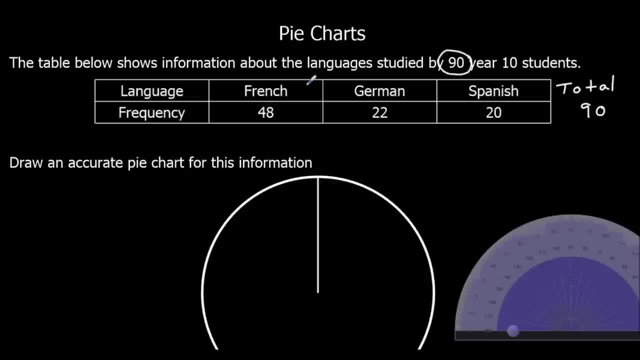 To draw a pie chart, we need to know that all the angles around the point, all the angles in the circle, add up to 300.. 360 degrees. So I'll make a note of that here: 360 degrees, And that will always be the case. 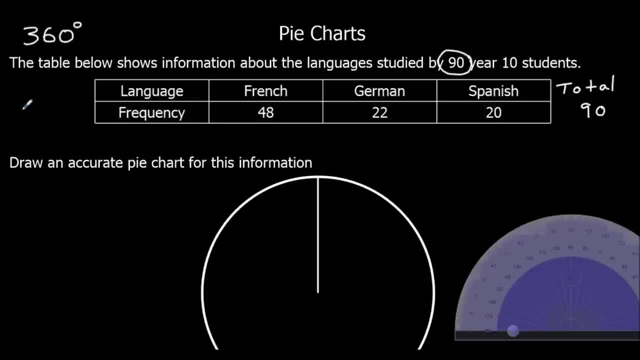 So in pie charts we've always got a circle, So it's always going to add up to 360 degrees. So we're going to have to work out what the angle for French, for German and for Spanish is. But we know the total angles must be 360.. 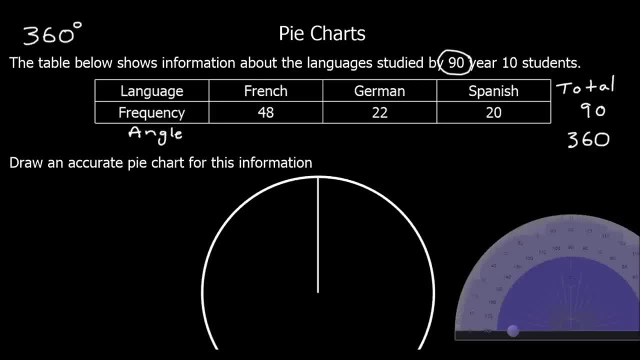 So what we do is we work out a multiplier. So how can we go from the frequencies to the angles? So we've got 90 in total and the angles 360 in total. So we're working out a multiplier. What do you multiply 90 by? 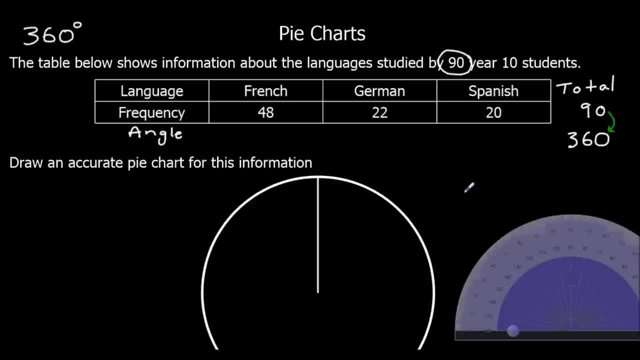 What do you times 90 by to get 360? How many 90s make 360?? And that's 4.. So we've got a multiplier of 4.. So to go from frequencies to angles, we are going to times by 4.. 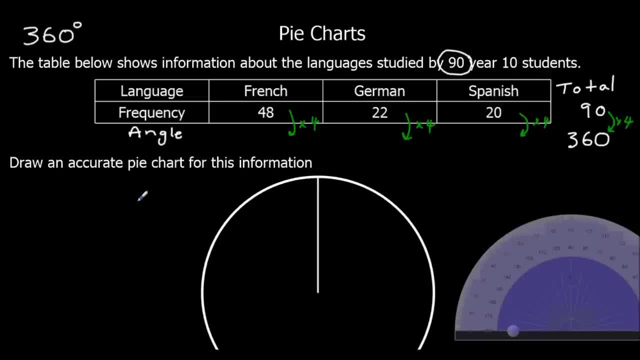 So we're going to do this for each of them. So for French, we've got 48 times 4,, which is 192.. For German, we've got 22 times 4. Which is 88. And Spanish 20 times 4.. 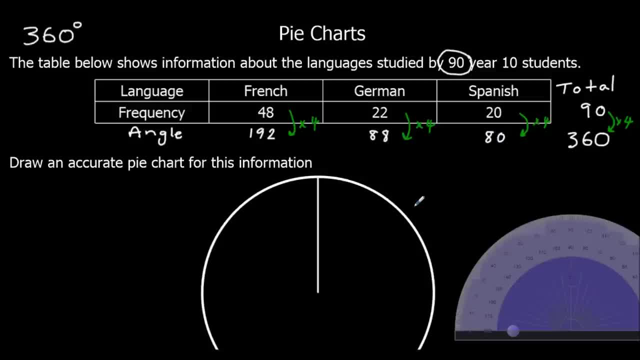 That's 80.. So here are our angles. We're going to draw 192 degrees for French, 88 degrees for German and 80 degrees for Spanish And if we add them up and check, we should get 360 degrees in total. 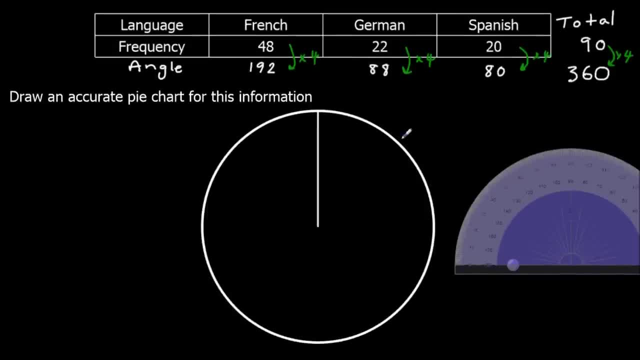 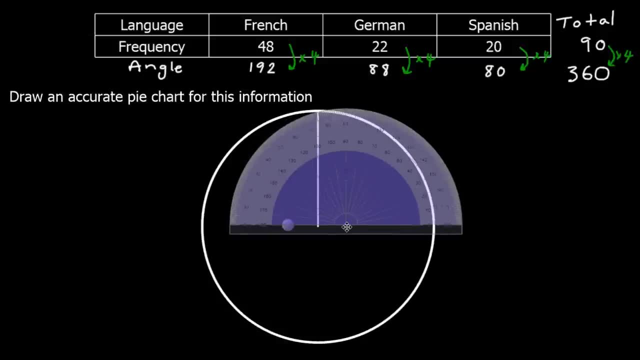 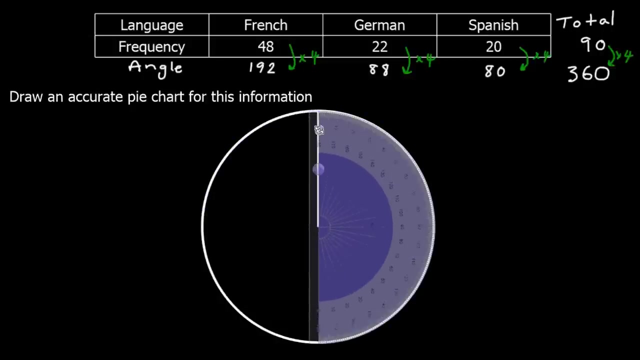 So let's look at drawing the pie chart. So we've got a protractor And we line up this part, the middle of the protractor, with the middle of the pie chart And we're going to spin it around. so zero starts on the line we've been given. 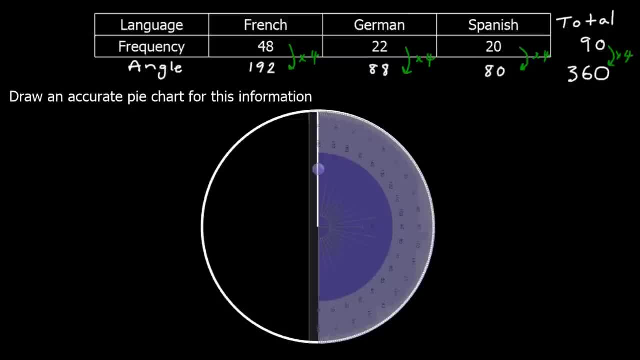 So we're going to start at zero And we want to go around to a hundred. So this is a protractor that only actually goes up to 180 degrees, So we need another 12 degrees, So 180.. We need 12 more degrees. 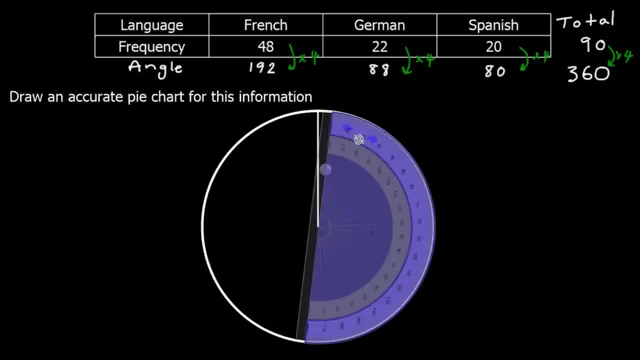 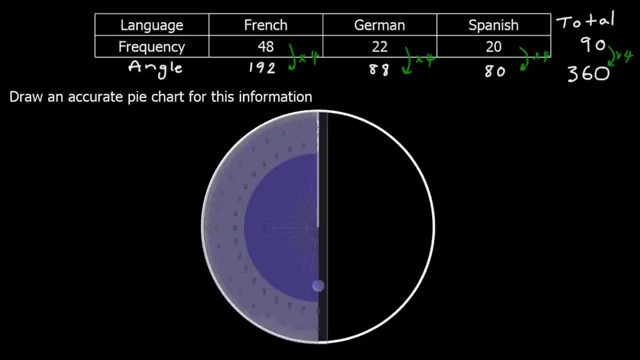 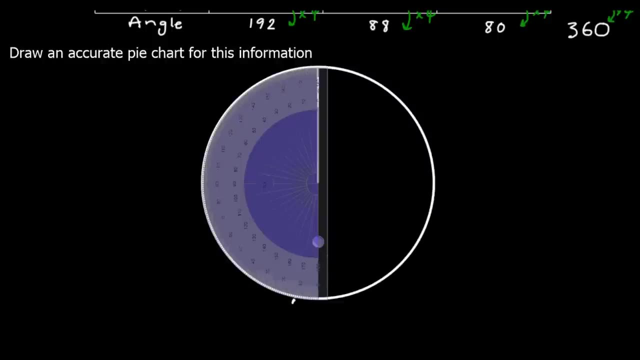 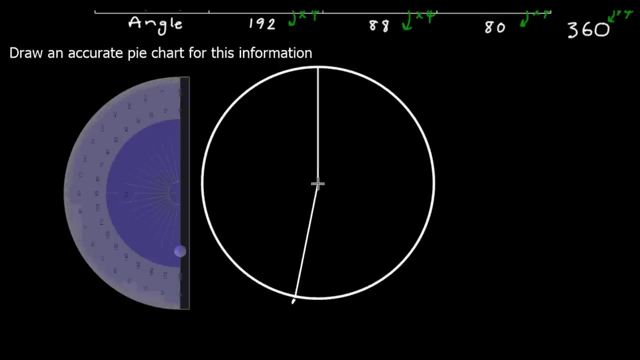 So what I'm going to do, I'm going to spin it all the way around. So I've got 180 degrees round to here, And I want another 12 degrees And I want another 12 degrees. So there we've got 192 degrees. 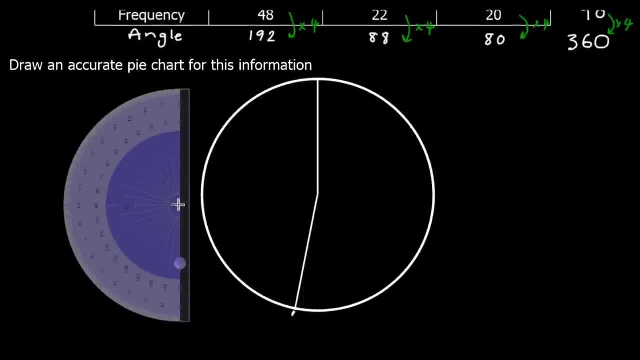 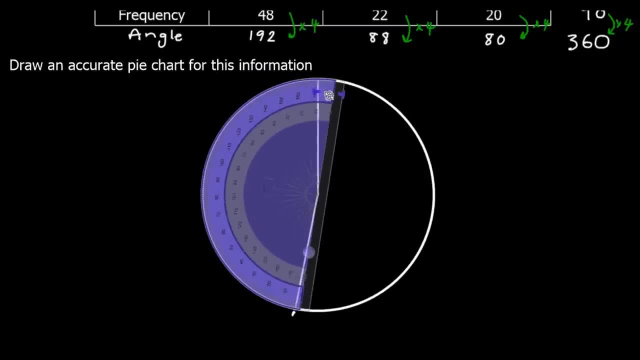 Now we want to measure 88 degrees. So again, the protractor on the center, We spin it around, So zero Is on the line, So zero is lined up And we want 88 degrees. So at zero we go up to 88.. 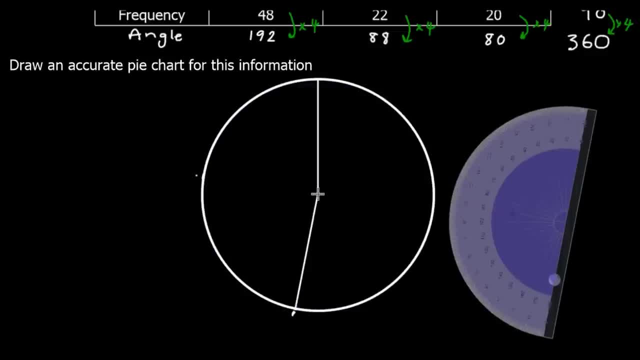 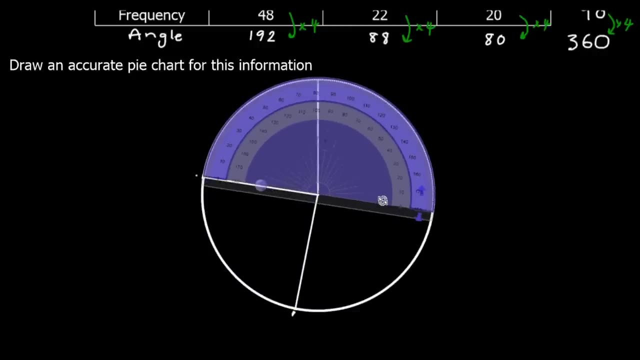 And we get our ruler And we join that line up, Then we should have 80 degrees left. So we can measure that. And we don't have any 80 degrees And here we have 80 degrees left. So now we just need to label our pie chart. 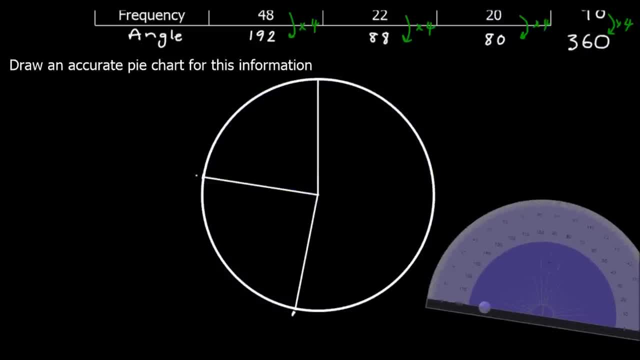 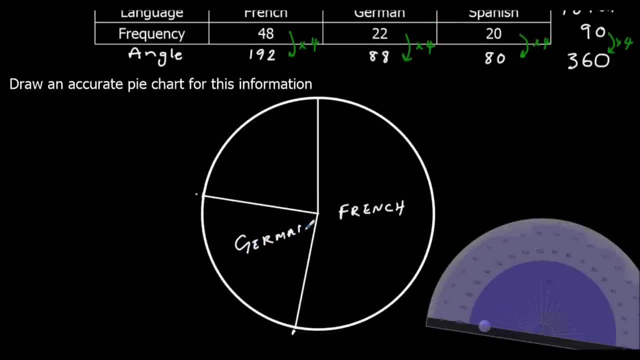 So we've got French, Which was at 192 degrees, Then we had German, Then we had Irish. So we've got that. We had English, We had Latin, We had Spanish, We had Spanish And we got Italian And we've got our blue here. 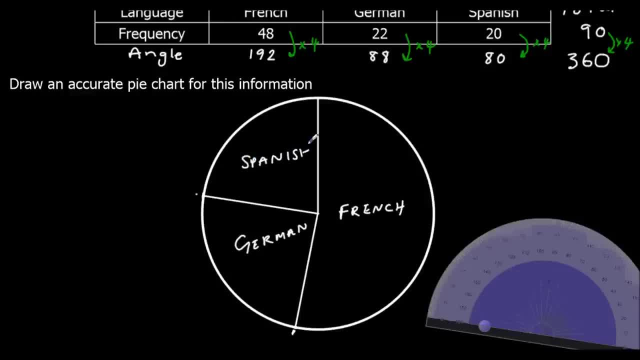 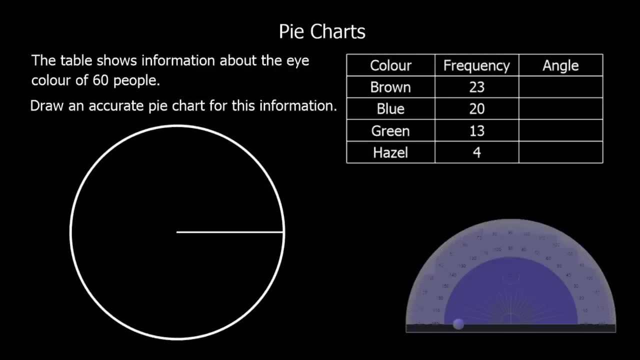 We've got our black, And we've got our purple, And we've got our yellow And we've got our orange And we've got our blue for 80 degrees. okay, here we've got another question. if you want to pause the? 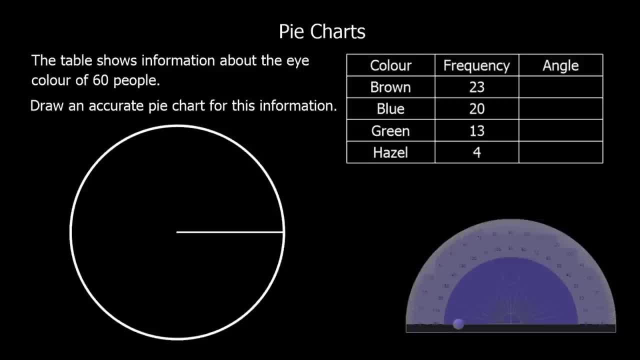 video and try and do this yourselves. you can otherwise just keep watching. so the question says: the table shows information about the eye color of 60 people. draw an accurate pie chart for this information. so again, we've got. we've got 60 people, so we'll add a total row in the bottom here and we've got 60. 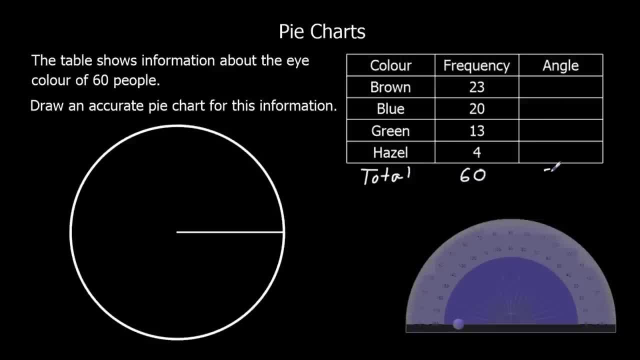 people in total and the angles in total have to add up to 360 degrees. so what is our multiplier this time? how do we get from 60 to 300 degrees? how many 60s go into 360? so we could do 360 divide 60 and that should give us an. 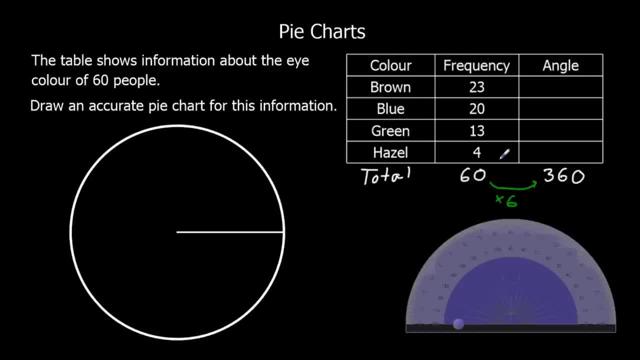 answer of 6. so our multiplier this time is 6. so we're going to times each of the frequencies by 6 to find out how many degrees they're represented by. so 4 times 6 can probably use a calculator for these um numbers, but 4 times 6 should give us 24.. 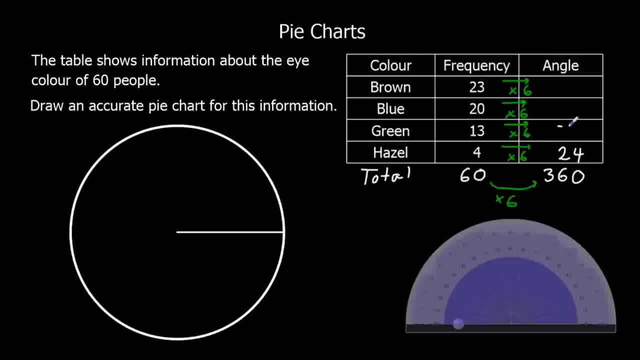 13 times 6 should give us 78, 20 times 6 is 120 and 23 times 6 should be 138. okay, so we've got our angles. we can check that. these numbers add up to 10 degrees, to 6 degrees. so 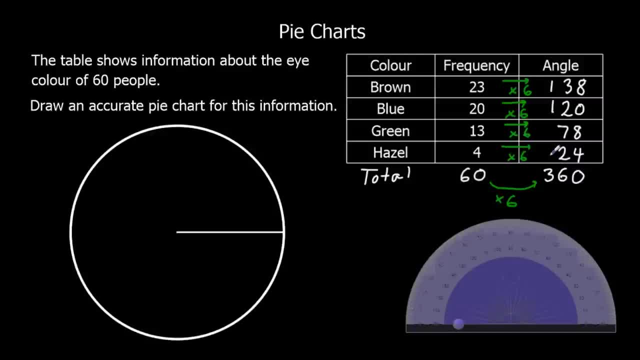 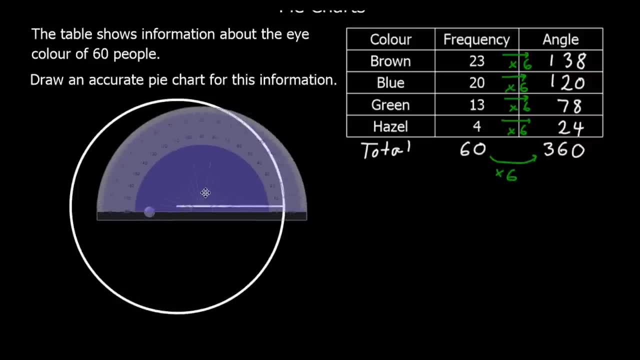 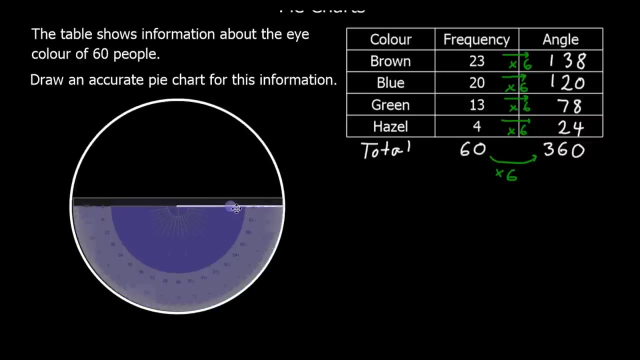 add up to 360, which they do. and now we're going to grab the protractor and draw these angles on. so we line up the center of the protractor with the center of the circle and I'm going to spin it around until zero is lined up with the 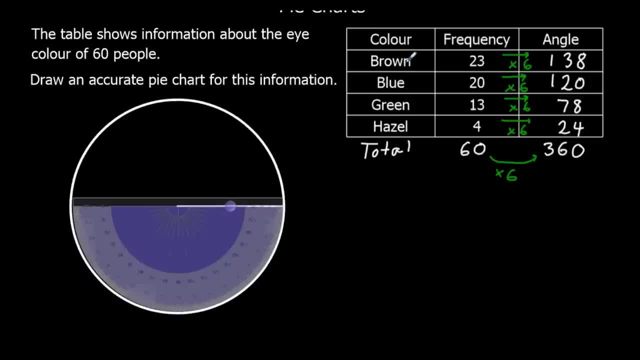 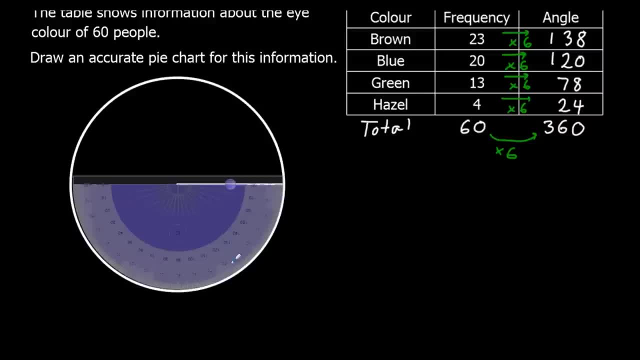 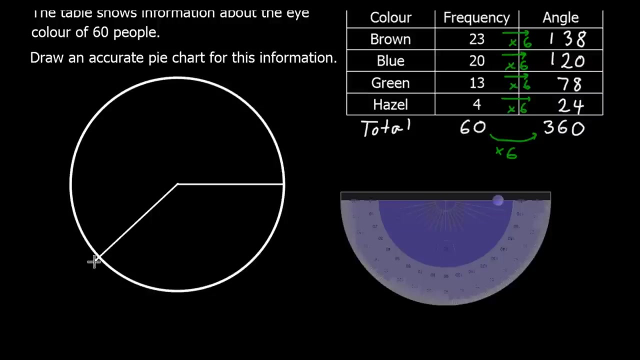 line we've been given. so we're going to do brown first, so we do a hundred and thirty eight degrees first, so zero all the way around to a hundred and thirty eight. then we're going to get the ruler and draw a straight line to complete the.